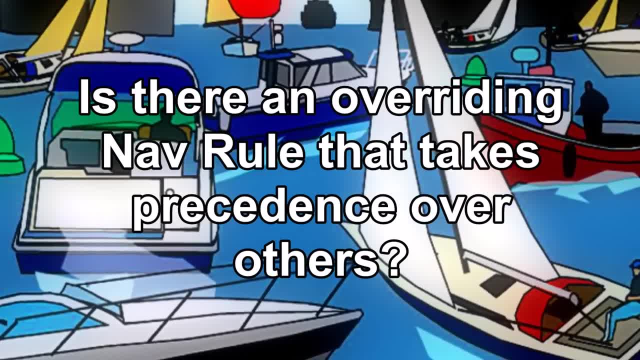 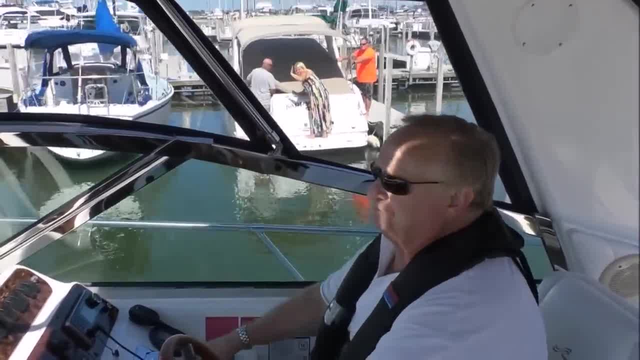 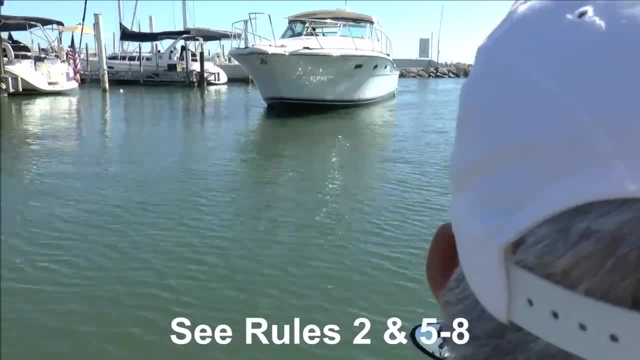 Is there an overriding nav rule that takes precedence over others? No, but there is a hierarchy for various situations, and all rules are focused on keeping vessels from colliding with each other, so each boater needs to know that he or she has a responsibility. Rule 2, Responsibility states In construing and complying with these rules. 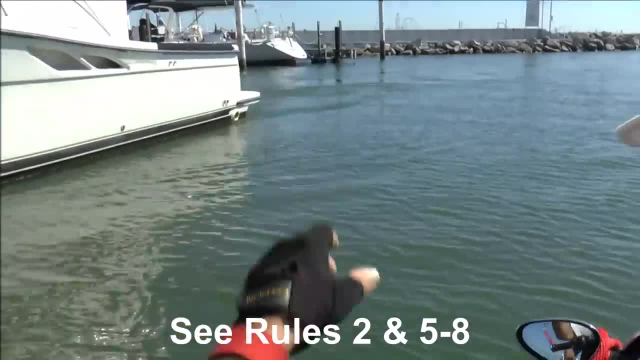 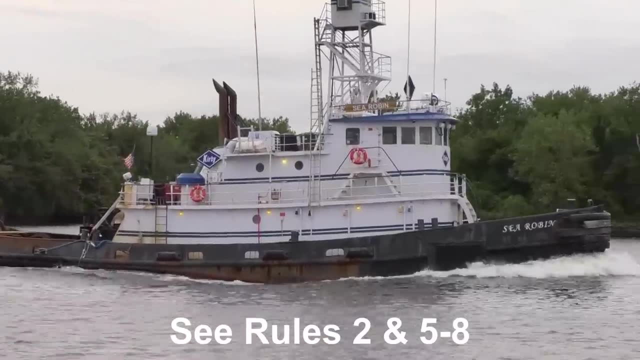 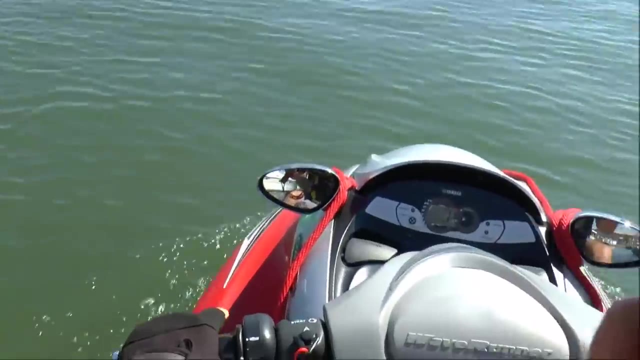 due regard shall be had to all dangers of navigation and collision and to any special circumstances, including the limitations of the vessels involved, which may make a departure from these rules necessary to avoid immediate danger. Nothing in these rules is required to comply with. rules shall exonerate any vessel or the owner, master or crew thereof from the consequences of. 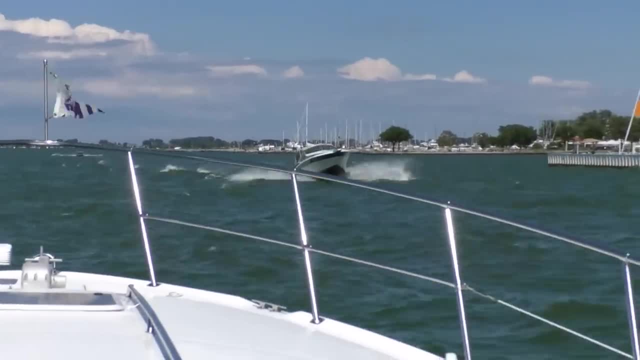 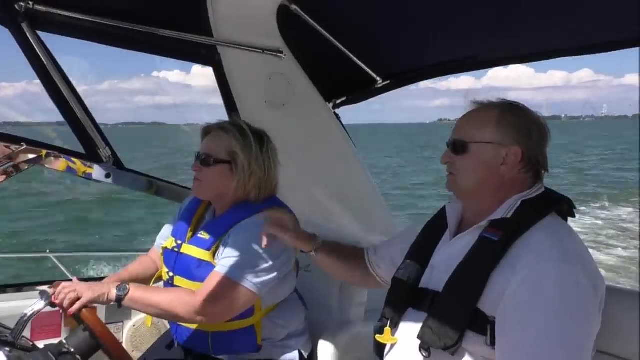 any neglect to comply with these rules, or of the neglect of any precaution which may be required by the ordinary practice of seamen or by the special circumstances of the case. Neglect, among other things, could be: not maintaining a proper lookout, use of improper speed, not taking the appropriate 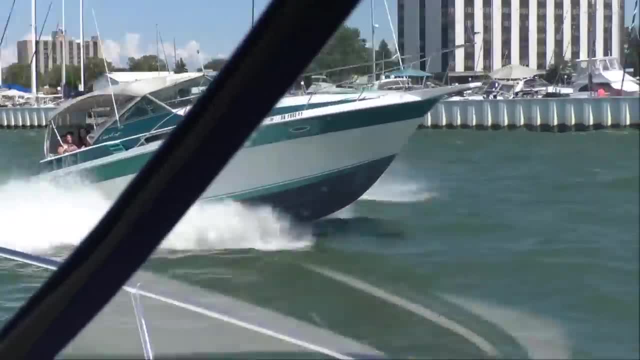 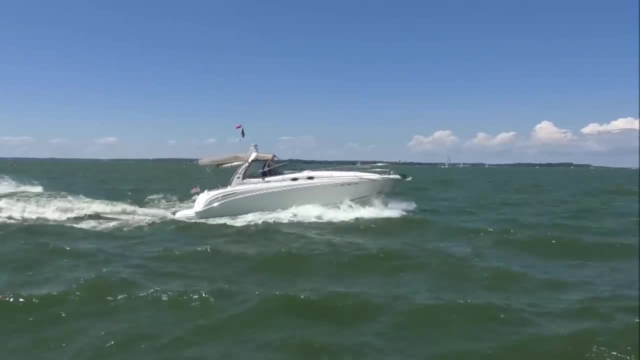 actions to determine and avoid collision or ignoring a boat operator's responsibilities. under the rules. No one has the right of way on the water. No one has the right of way unless Rule 9 applied. Good seamanship suggests that operators should know the limitations of the vessels involved. 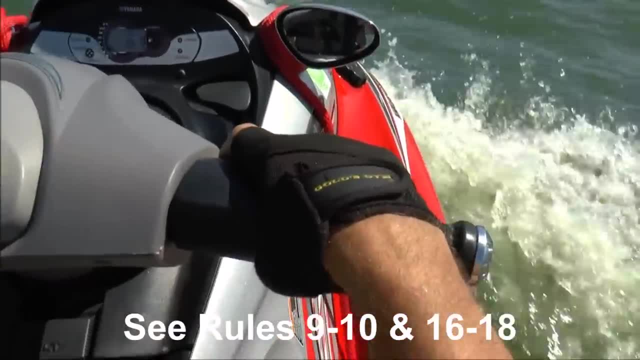 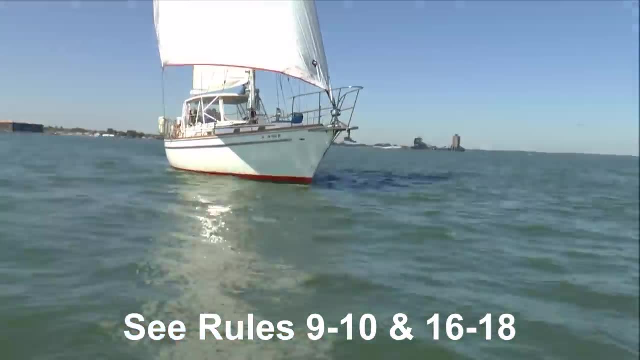 to avoid immediate danger. Power-driven vessels, which are defined as any vessel propelled by machinery, regardless of whether the machinery is being used, are to keep out of the way and, depending on circumstances, either give way, meaning move aside, or slow down or stand. 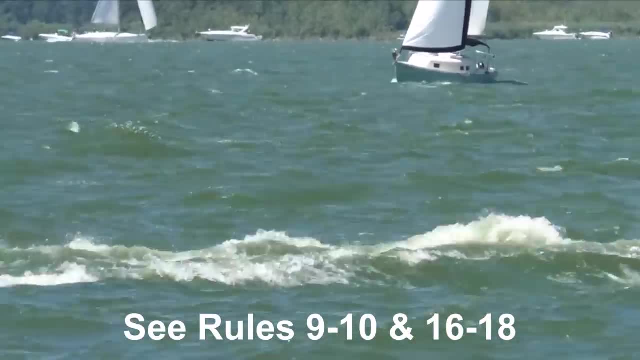 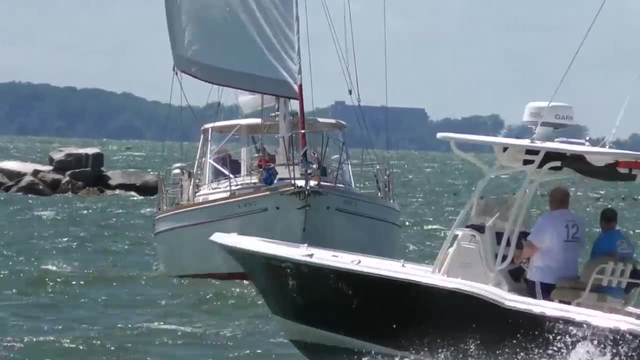 on meaning not change course with respect to vessels not under command. Vessels under command are restricted in their ability to maneuver sailing vessels or vessels engaged in fishing. Similarly, vessels should avoid impeding the safe passage of a vessel constrained by her draft or navigating a. 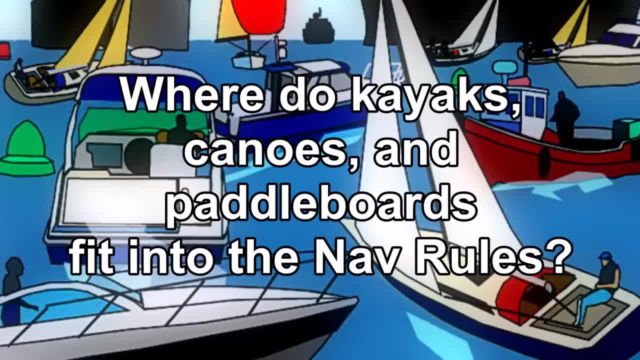 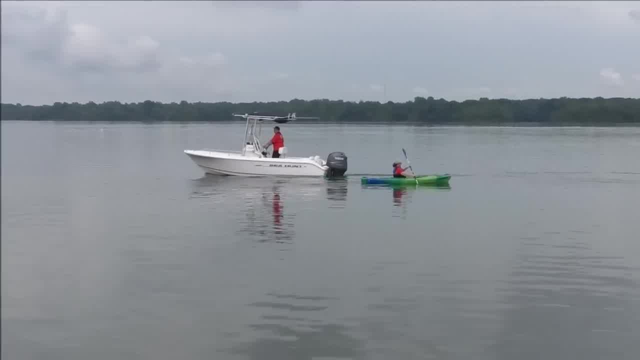 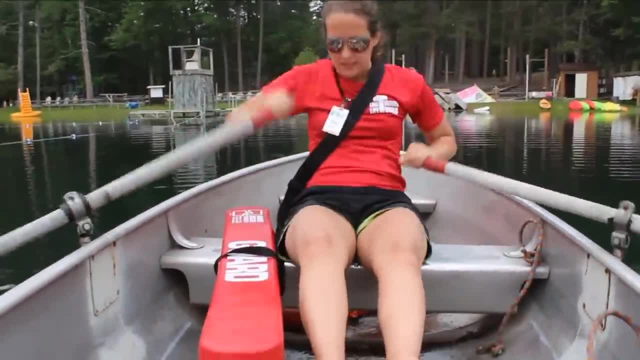 narrow channel or traffic separation scheme. Where do kayaks, canoes and paddle boards fit into the NAV rules? They must also follow the NAV rules as they are also vessels. Kayaks, canoes, paddle boards and other such human-propelled watercraft are considered to be vessels under oars. 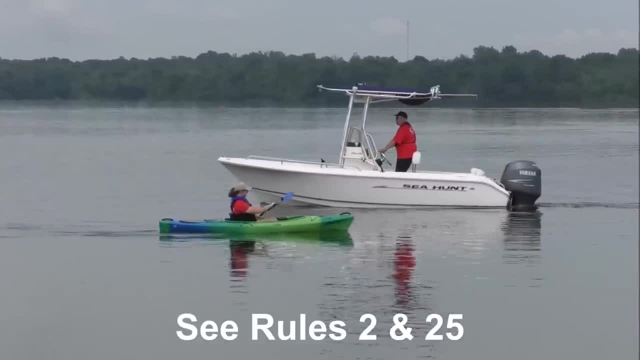 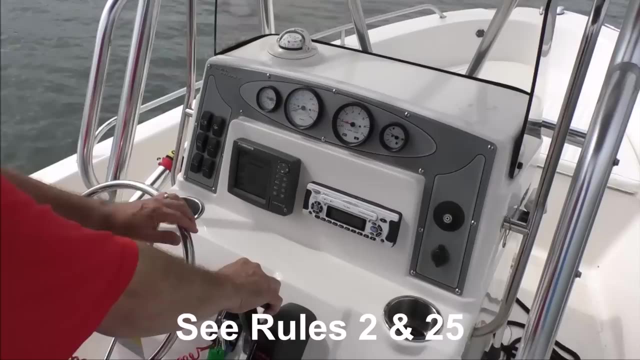 What would be required by the ordinary practice of seamen or by the special circumstances of the case, determines whether a vessel under oars is the give way vessel meaning- it must slow down or move aside when approaching another watercraft- or the stand on vessel meaning. 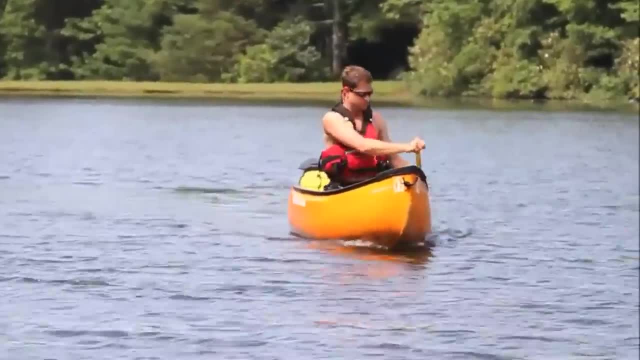 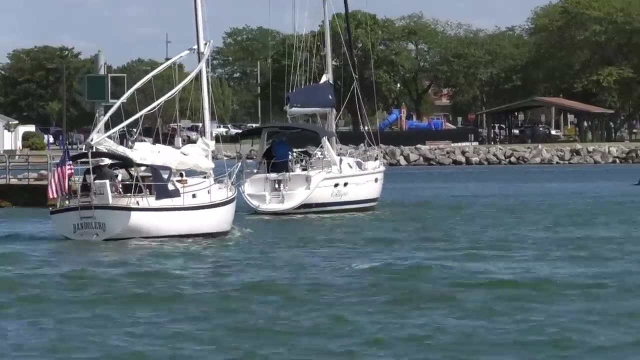 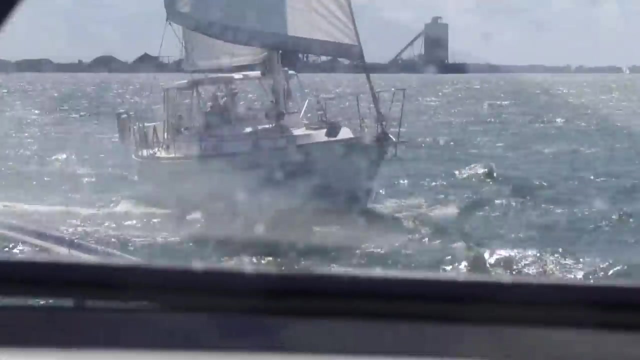 it must maintain its course and the notion that they are less able than most other vessels. What is the safe speed or passing distance for vessels When crossing, meeting or overtaking another vessel? as the boat operator, you must keep your vessel well clear of the other vessel. 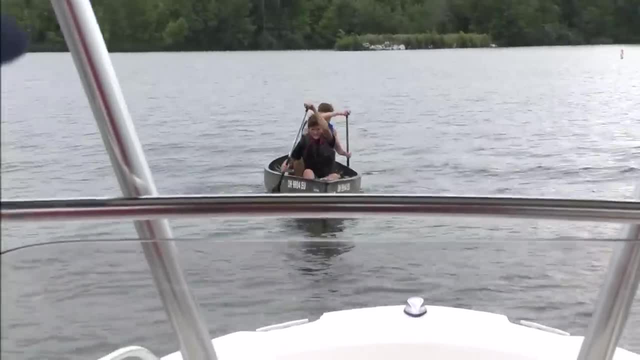 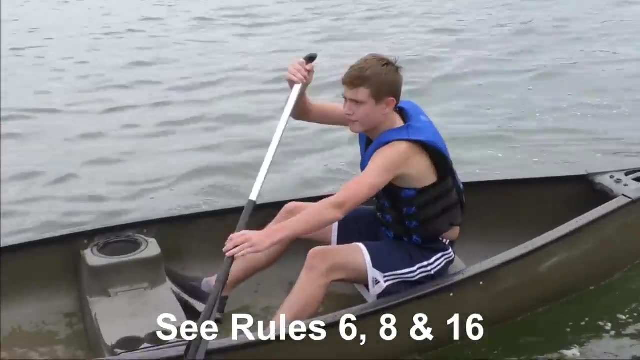 Similarly, the distance required for a vessel to take action to avoid collision will vary. However, it should enable doing so at a safe speed to avoid a collision. Any alteration of course or speed shall be large enough to be readily apparent to another vessel. 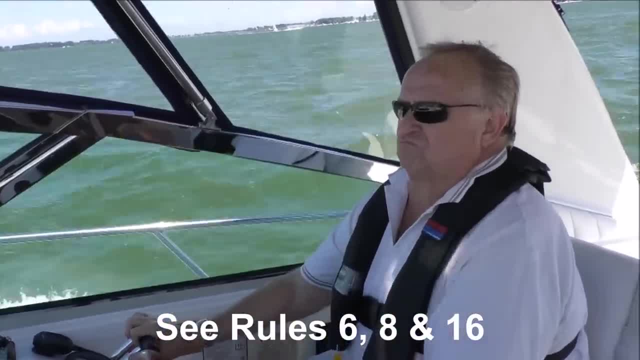 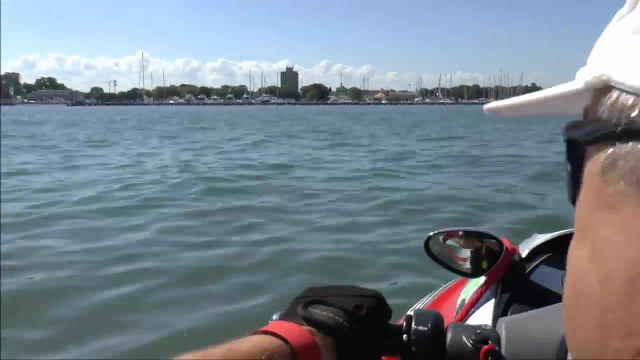 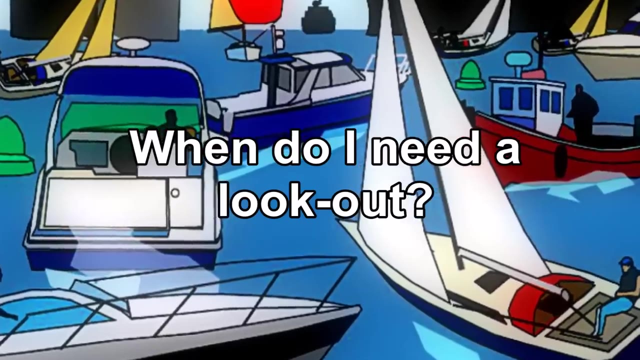 Such alterations shall be taken early enough and be stopped within an appropriate distance to allow sufficient sea room for the safe passage of the other vessel at a safe speed. The alternation will be complete at the same time, All vessels are responsible for maintaining a proper lookout at all times. 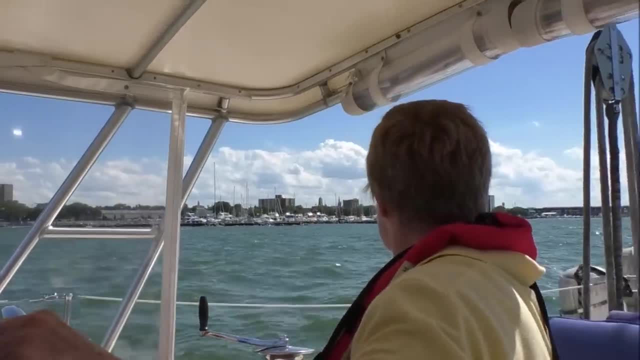 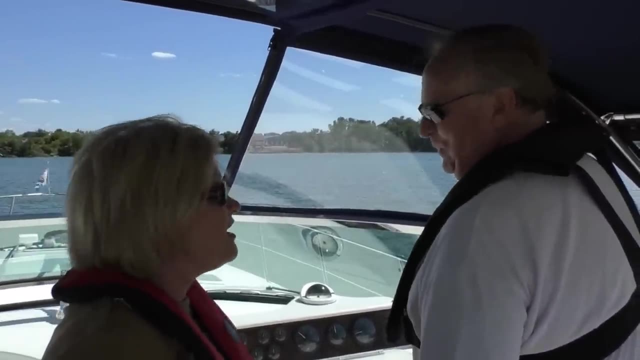 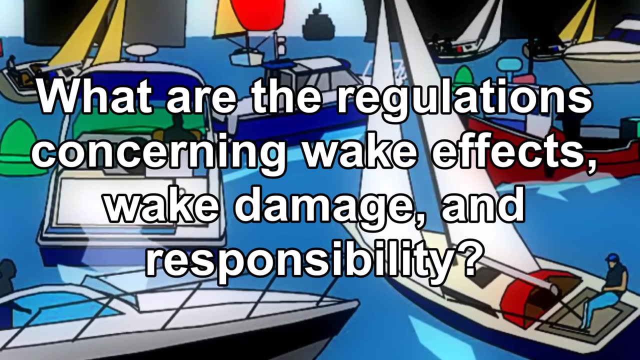 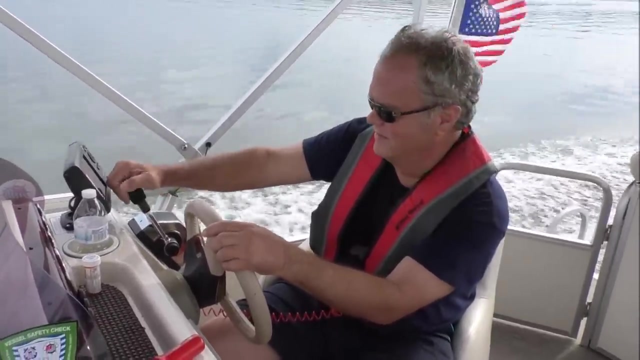 This includes one-man crews and recreational boats. The term lookout implies watching and listening to be aware of what is happening around the vessel. The emphasis is on performing the action, not on the person. What are the regulations concerning the vessel? Recreational vessels are required to operate in a prudent manner that does not endanger. 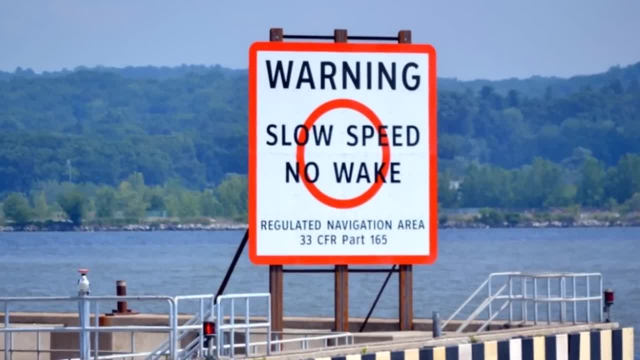 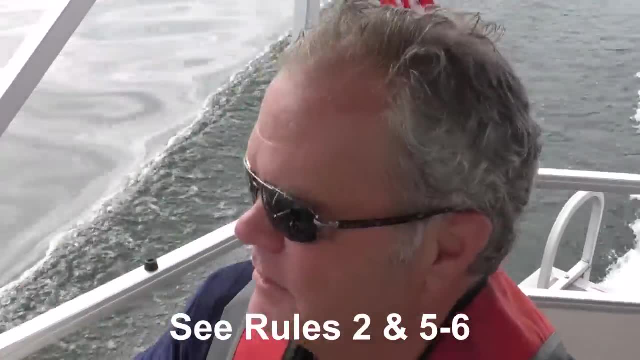 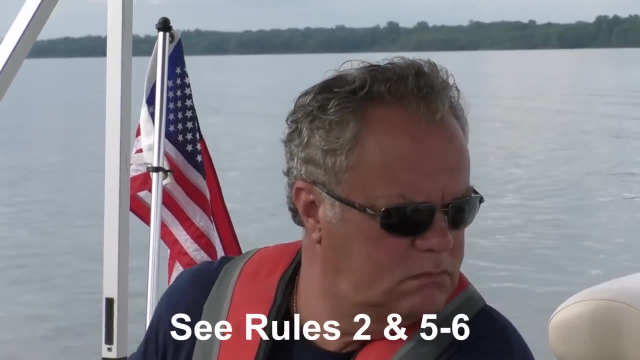 life, limb or property. There may also be state or local laws which specifically address weight for the waters in question. The NAV rules do not exonerate any vessel from the consequences of neglect which, among other things, could be unsafe speeds, improper lookout or ignoring prescribed responsibilities. 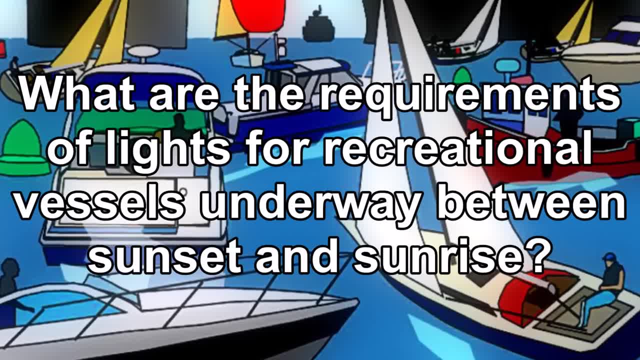 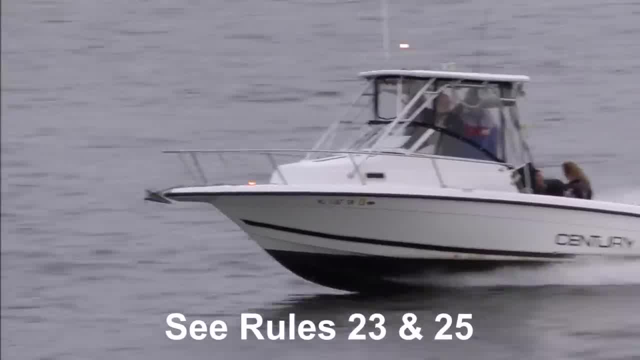 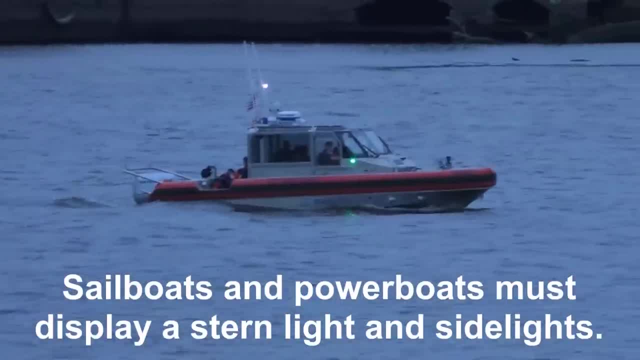 under the NAV rules. What are the requirements of lights for recreational vessels? The NAV rules require that the vessel operate in a prudent manner that does not endanger life, limb or property. What are the requirements of lights for recreational vessels? A light can be on either one of the vessels that the person is sitting in. 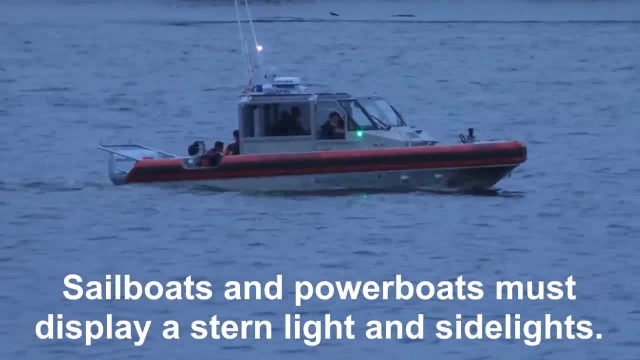 On the bottom of the vessel there is the LED which is the wind disciplined ihn for 瞬 кап to indicate of the wind. The LED indicates that the vehicle is not on a sidewalk and the light is on the left hand or port side of the vessel. 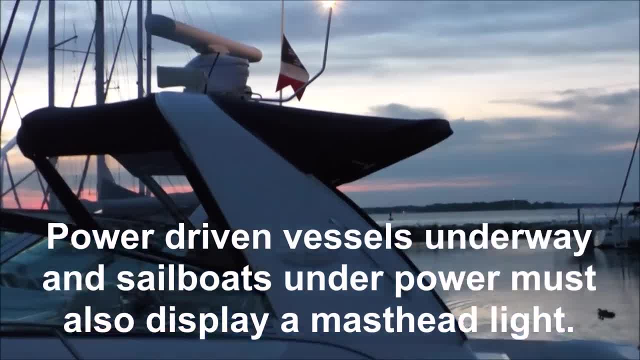 The force of the light depends upon how large the water is In the right hand or starboard side of the vessel the power being set off. there is a green light on the outside direction, which may be a people's light. The blue light indicates the direction in which the person is piloting the boat. The red light indicates the direction in which the person is piloting. The light will be mixed with the other lights in the 그런데. Power driven vessels or 39.4 feet in length and sailboats must at a minimum exhibit a white light.